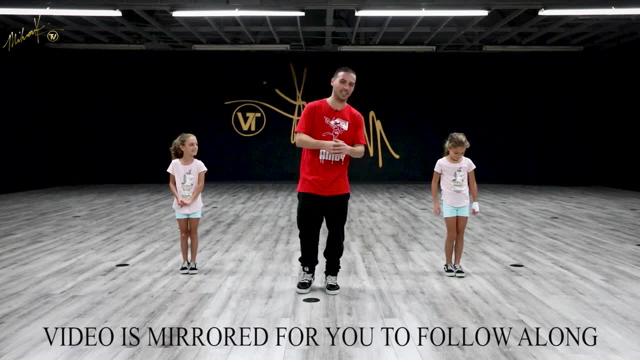 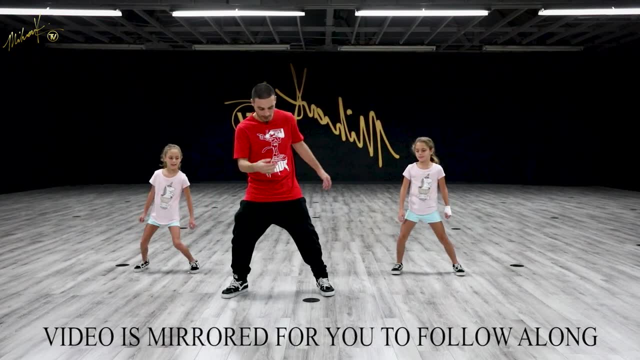 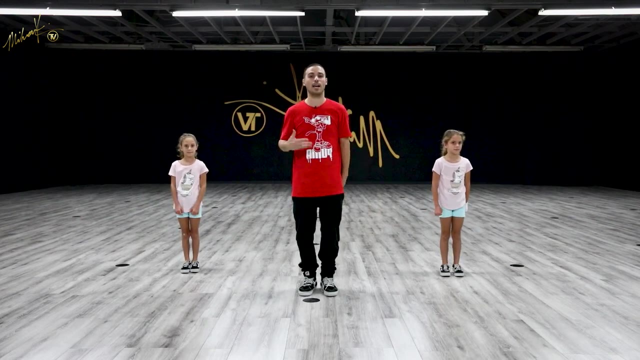 hello Lily. All right, you guys ready, Ready? All right, let's get started. Here we go: Right leg together, left leg together, right leg together, left leg together. Good, You just want to make sure you're bouncing every time you step, so just put a little bounce to your step. 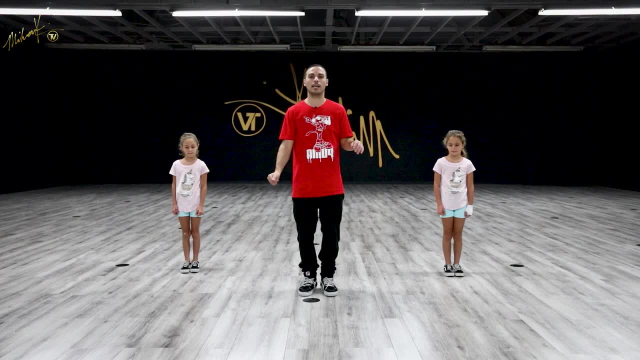 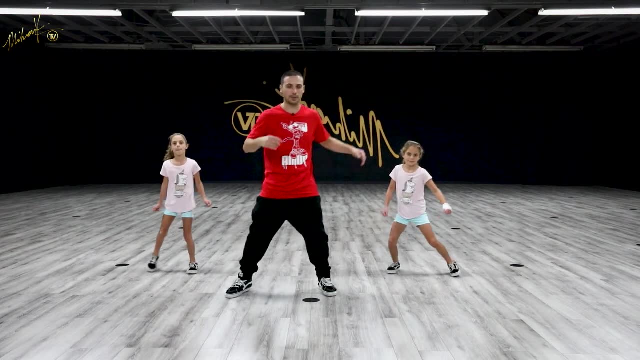 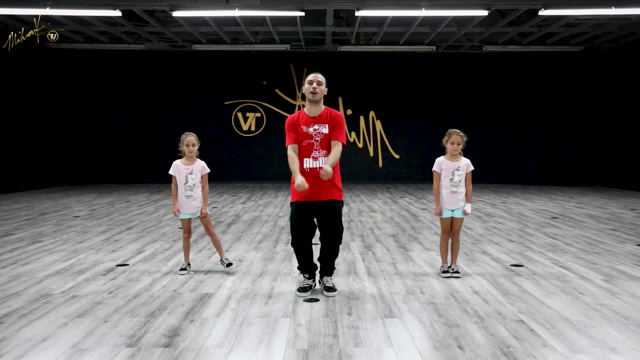 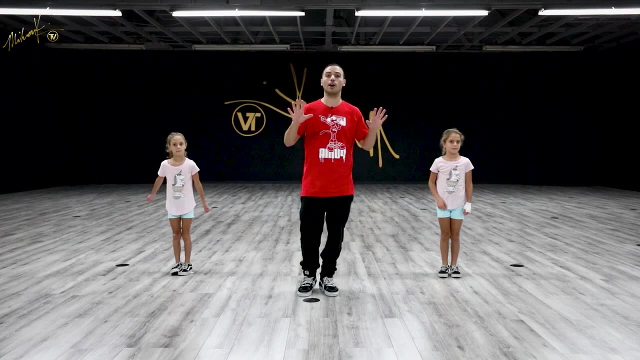 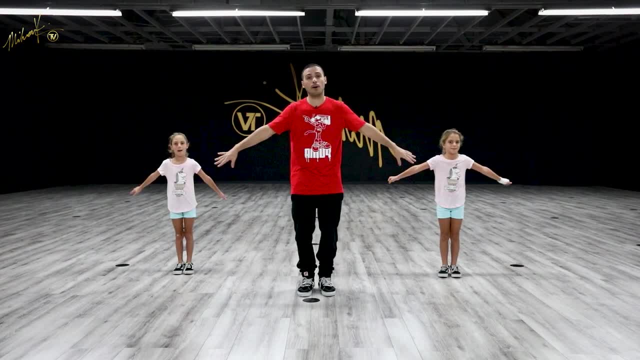 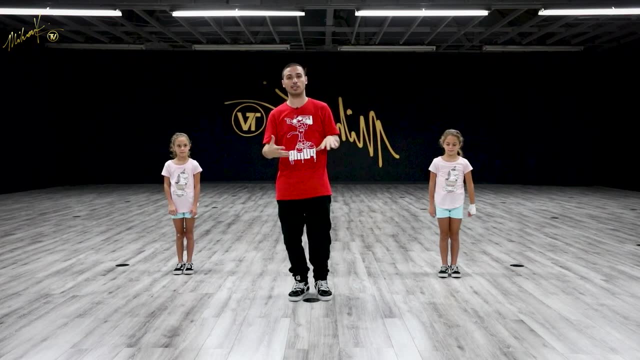 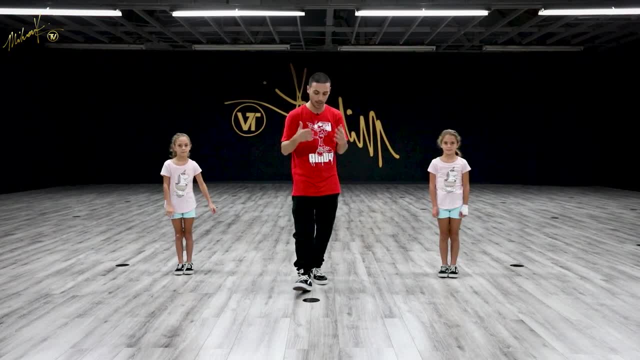 you step out and when you come together, you're going to clap at the same time, okay. Every time your feet are together, you're going to clap at the same time, okay. So let's do it one more time. We're clapping, Let's try again. Just the arms- Five, six, seven, eight- Go out and clap out and 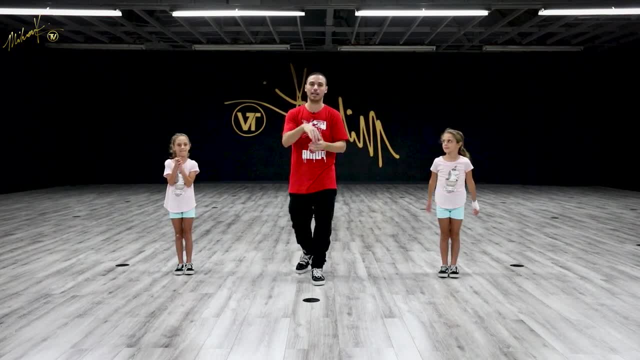 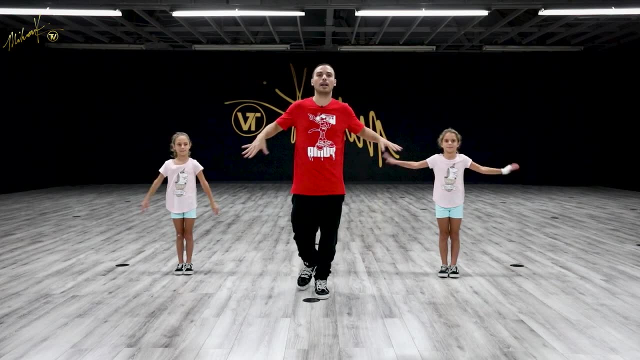 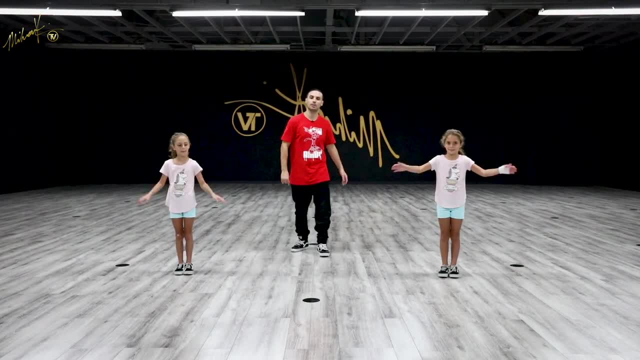 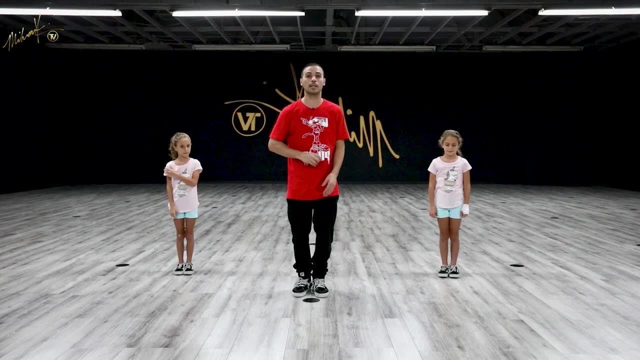 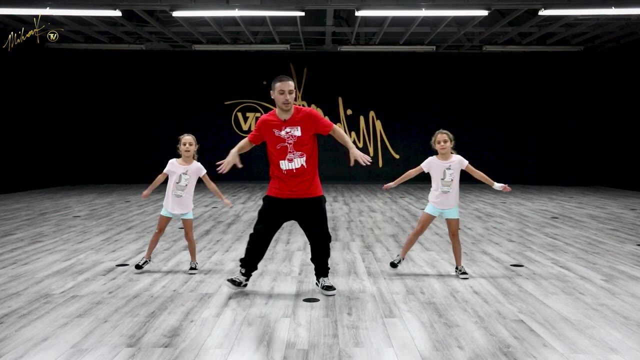 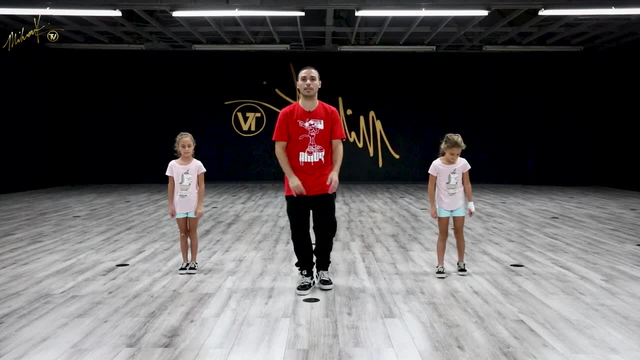 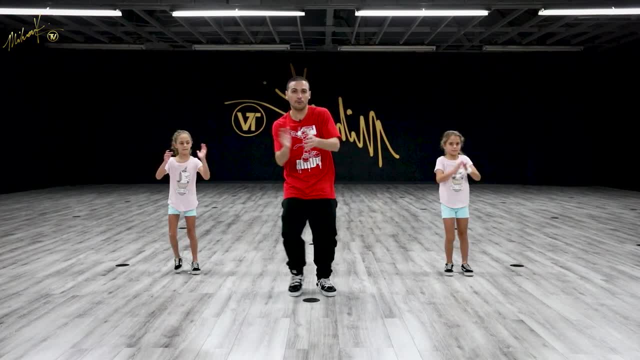 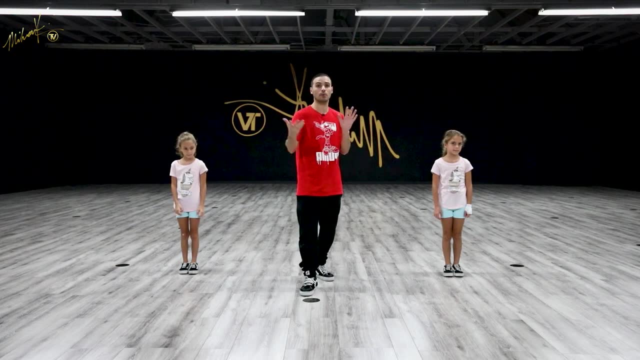 seven: go One, two, three, four, five, six, seven, eight. Good, Moving on from here, We're going to step out with the right leg, We're going to turn our body, We're going to go one feet. go out, bring the feet back. 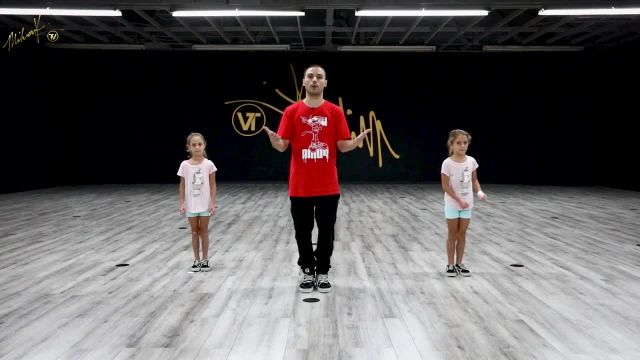 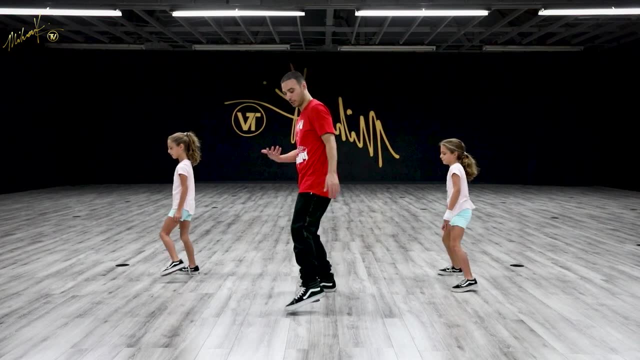 two go again. three turn back around four. Good, One more time just for the feet. A couple more times. Here we go: Six, seven, eight. Step out with the right leg, Bring the right leg in. 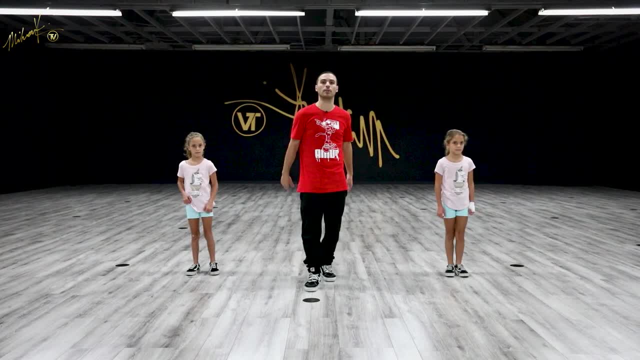 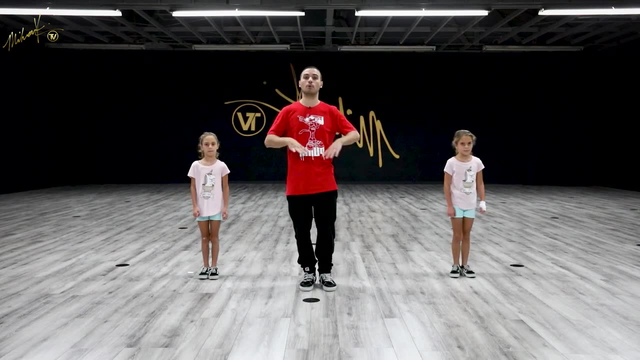 out again, Turn your body back to the front. Here we go. Five, six, seven, eight, Go out and in and out and turn. Good, We want to make sure we keep that same balance again. Okay, So let's do it with the bounce girls. Six, seven, eight, Go one. 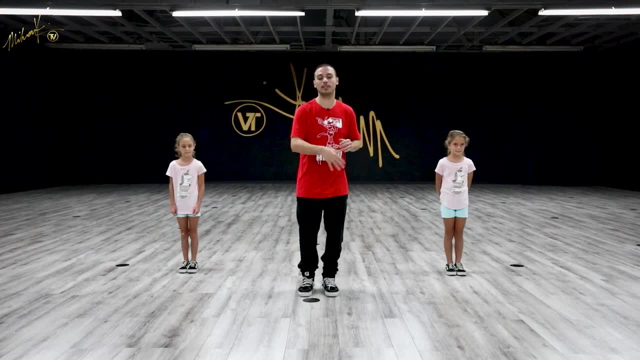 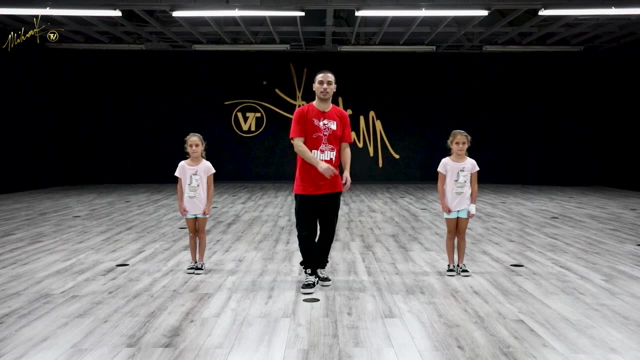 two, three, four Good. Six, seven, eight Step out in out turn Good. One more time. Five, six, seven, eight Go out in out, turn Good. We're going to keep that balance every time I'm. 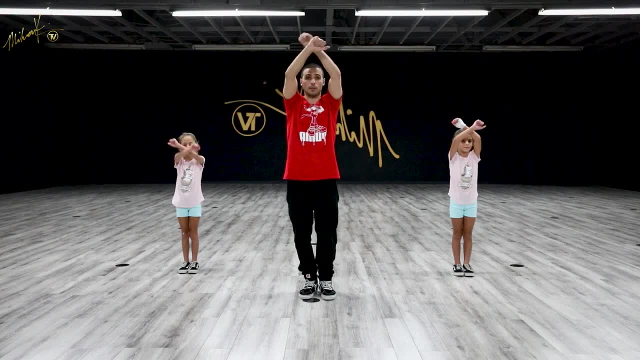 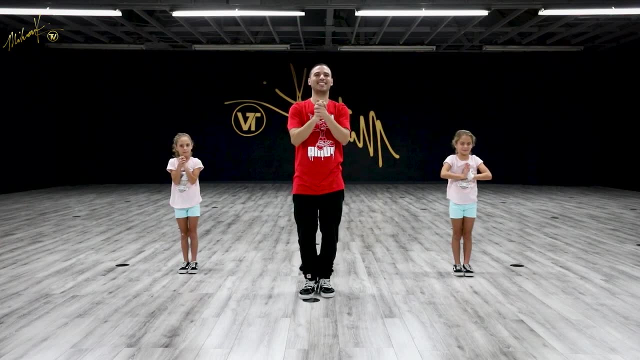 going to show you guys the arms. now Let's go, girls, Arms out and cross and out and clap. Okay, Clap, Sophia, Six, seven, eight, Go out, cross out, clap, Awesome Again. Five, six, seven. 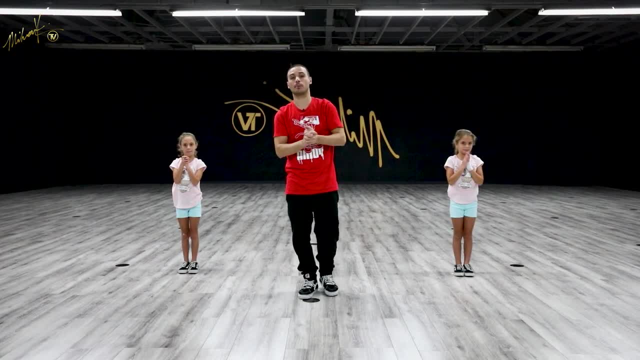 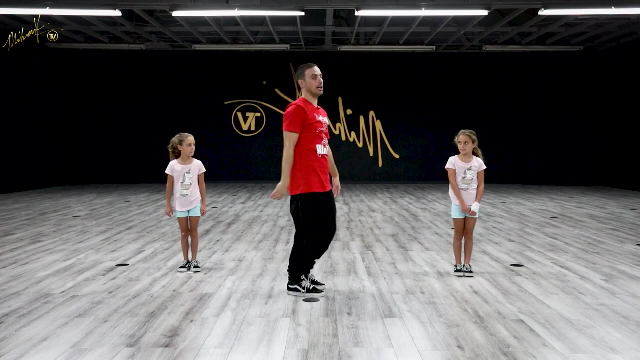 eight, Go out, cross out, clap, Awesome. Make sure the arms are above your head so you are not covering your face, and then bring it down. Okay, Now, with that I'm using my body a little bit, So if you see me standing profile, I have a little rock with my body. So that's going. 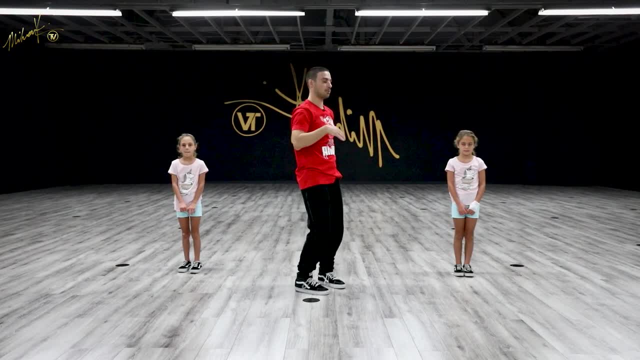 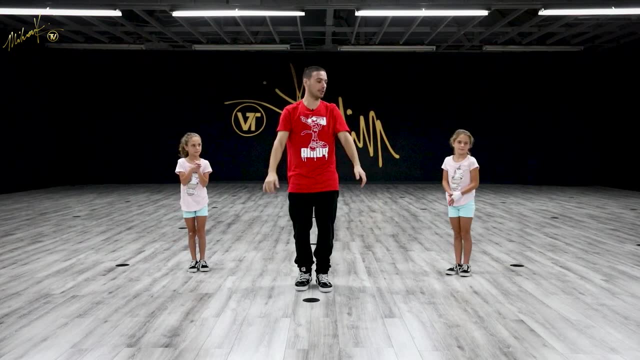 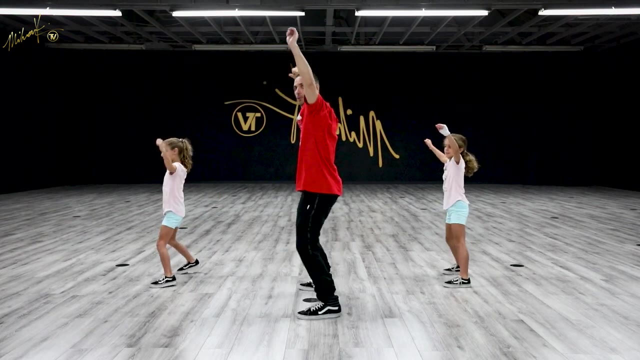 to help you really move. So you don't want to be stiff like this. Okay, So just push your body forward just a little bit as you step, step, step, clap. Let's do it slow, girls. You ready. Here we go, Five, six, seven With the arms. we're going one, going two, going three, clap. 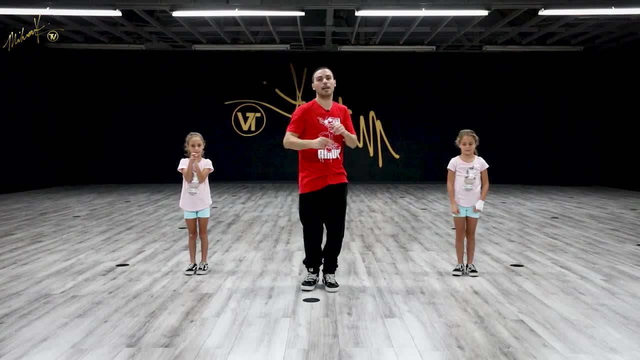 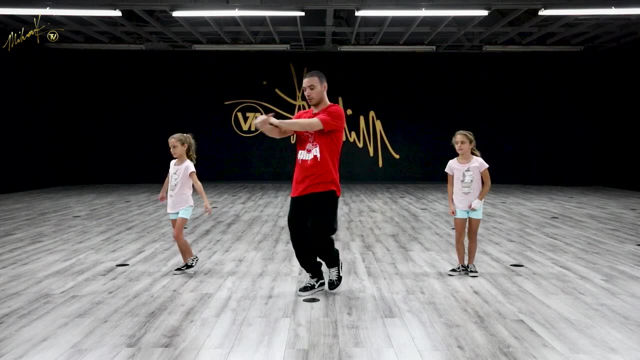 four Again, Five, six, seven, eight. Go one, go two, go three and clap Four Good Again. Six, seven, eight. Go one, go two, go three and clap Speed it up. 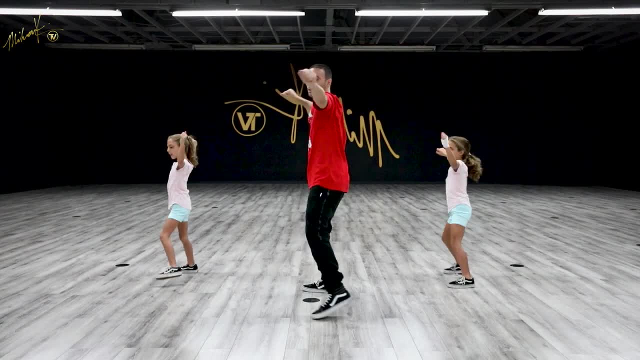 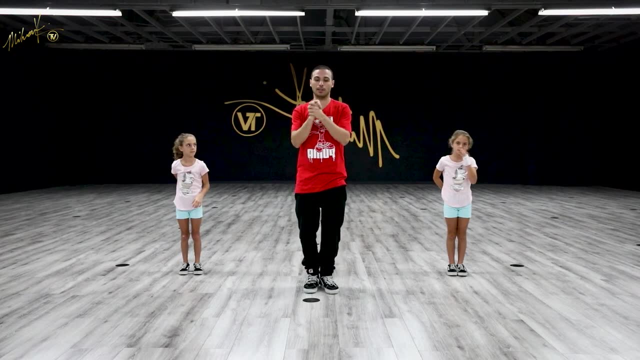 Six, seven, eight, Go one, go two, go three and four. Good, Right from here we're going to. pretty much it's going to look like we're about to do the same thing on the other side, because we're going to step five. but we're not going to continue, We're just going to lean over Six. 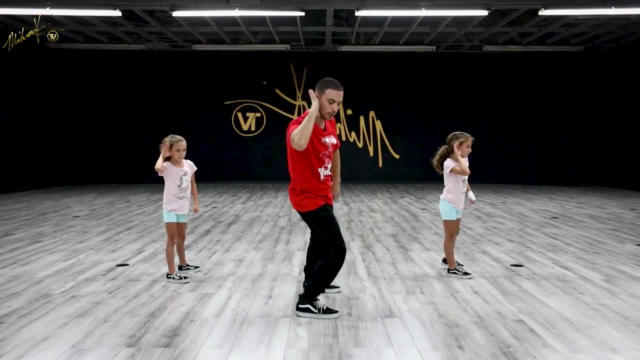 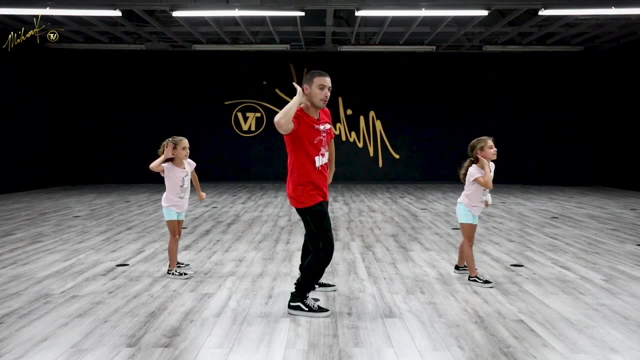 like we're about to hear something and we're just going to go. seven, eight, Okay, Super easy. So we're here, We just clap Right, girls, We're going to turn on five. We're going to lean over. The arm goes behind the ear. 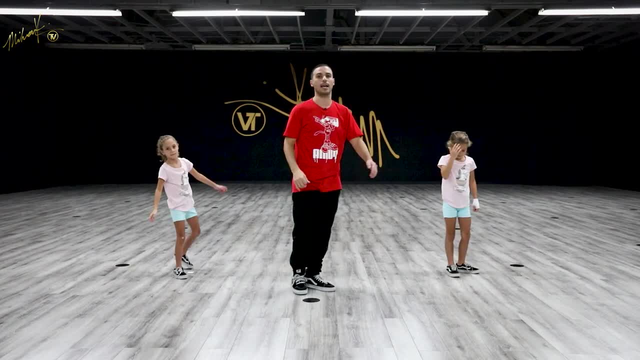 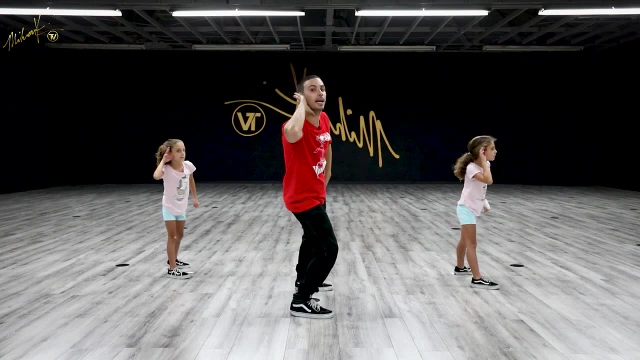 and then we're going to go and down and down- Good. Again. Three and four, step five, lean six and down and down- Good. So I'm going to give you the counts for that part one more time. 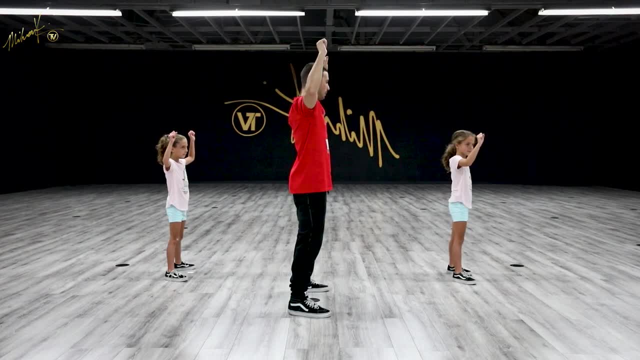 so you remember Five. we step and the arms are up. Right, Sophia, Arms are up and then we're going to lean. So just the lean and the ear, That's six. So you don't want to be leaning. 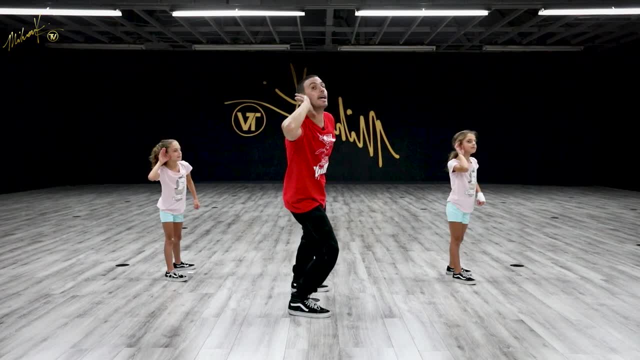 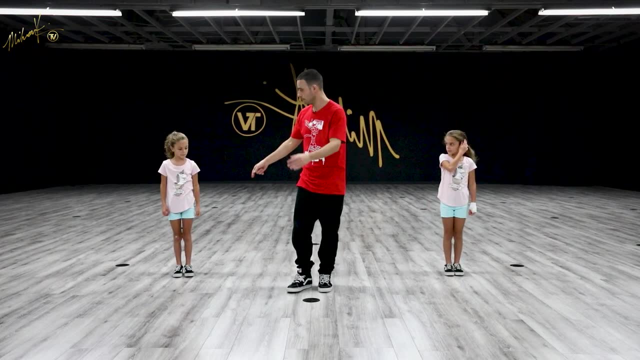 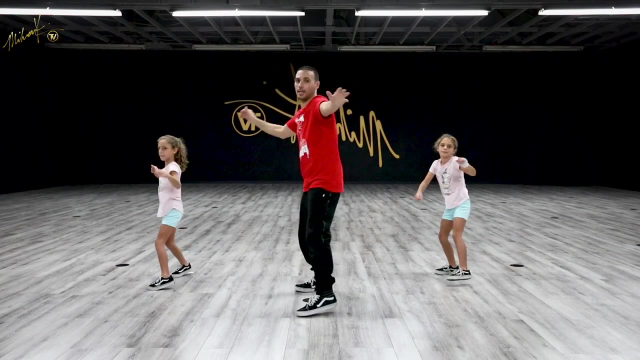 and you don't want to move your head yet. Your head is going to come right after It's going to go. and seven and eight, Okay, So let's do the part before that and connect it together. You ready, Ready, Soph, Here we go. Six, seven, eight: Step one and a. two. three and clap, Step five. 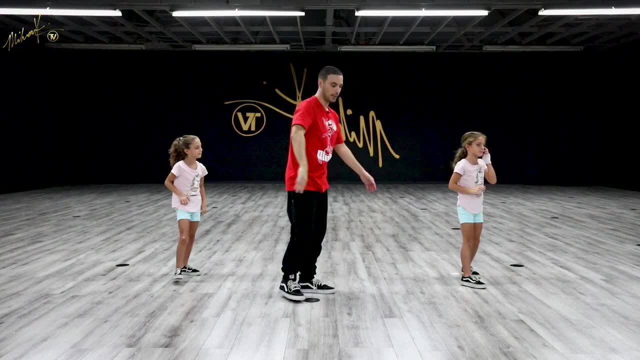 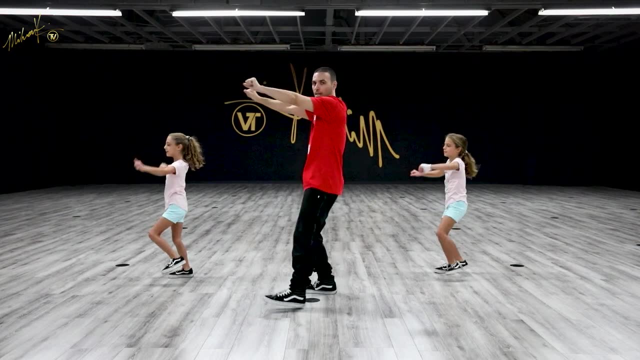 lean six up down, up down. Awesome, Here we go again. Just a little bit of speed: Five, six, seven, eight, Step one, step two, step three, clap four and arms lean up, down, up down, Good. 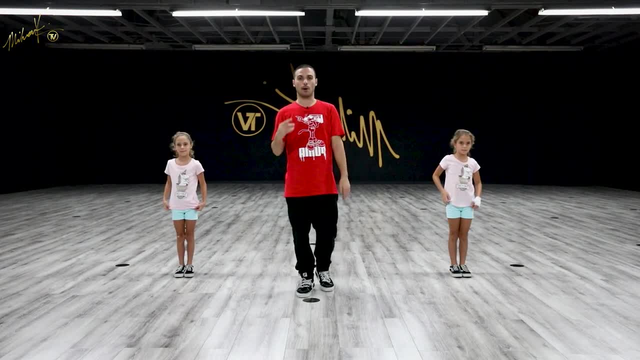 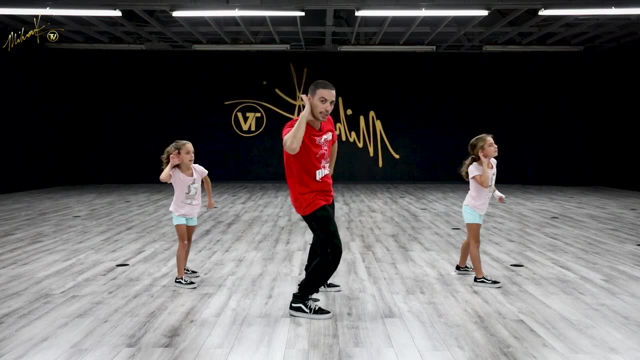 One more time and then we're going to go all the way back to the top. Here we go: Five, six, seven, eight, Step one, step two, step three, clap four, step five, lean six, seven, eight. 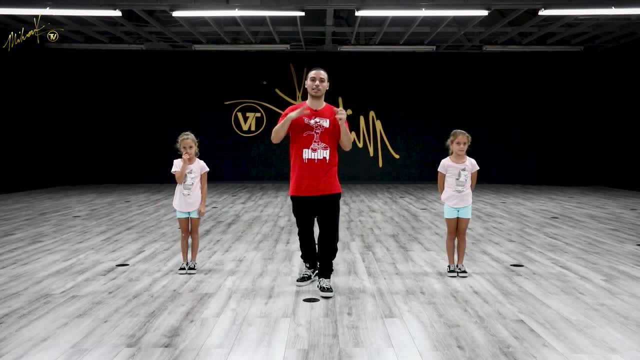 Awesome guys, Let's go back to the very top. Let's walk that whole thing slow and then medium tempo and then we'll do it with music. Okay, Here we go From the top, really slow, just to recap: Six, stepping out with the right arms out and then clap Seven. 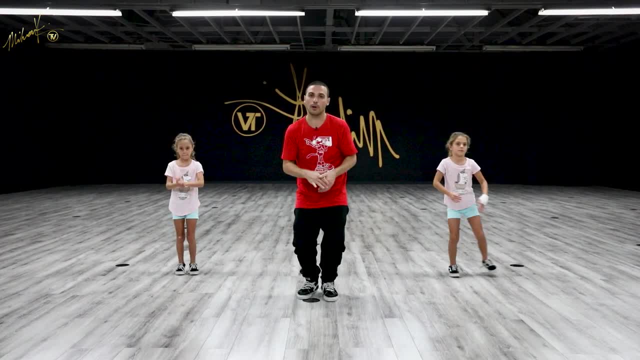 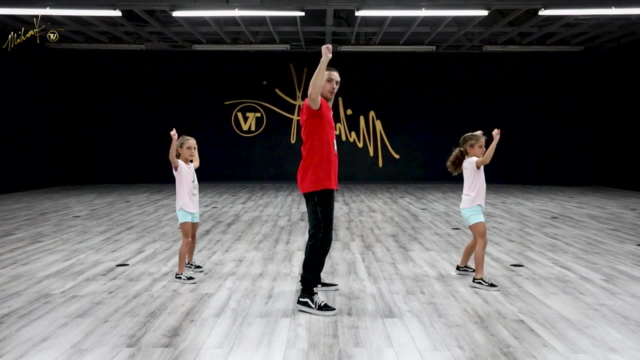 eight: We went one and two, three and four. Take your time, Keep the bounce, Go, step, go, step, go, step and clap, Boom, boom, up and up. Good, Again, here we go, A little bit more speed. Five: 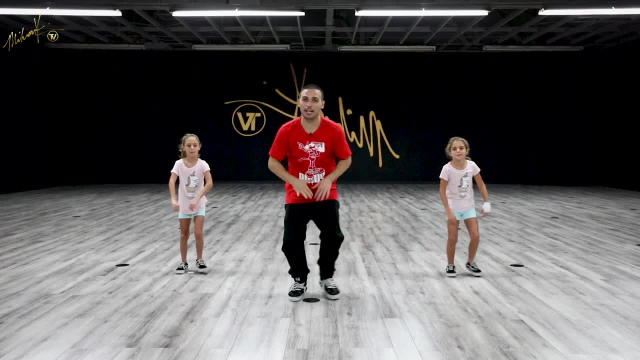 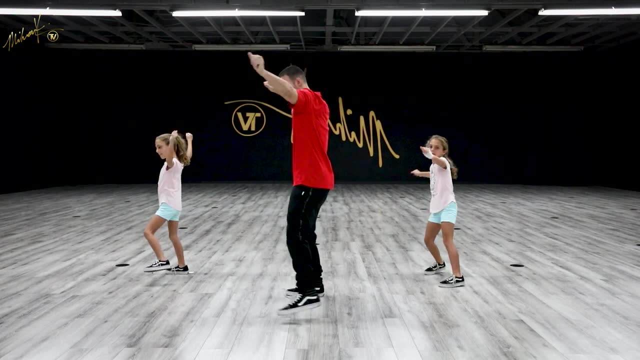 six, five, six, seven, eight. Go one, two, go three, four, go five, six, go seven, eight. Go one, two, three, four, five, six, seven, eight. Good, How do you guys feel? 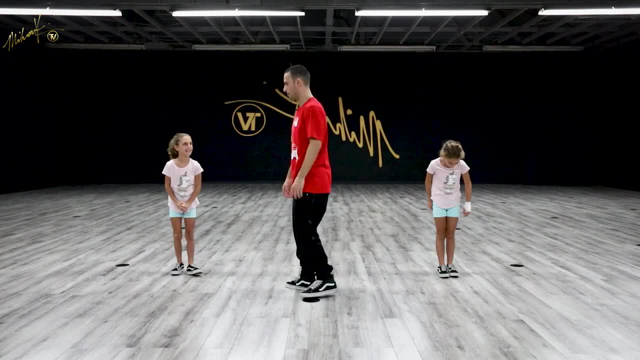 You feel good, Soph, Good for you. Yeah, Lily, Good for you. All right, let's do it again. Can we go a little faster? Let's go a little bit faster and then do it with music, with them. 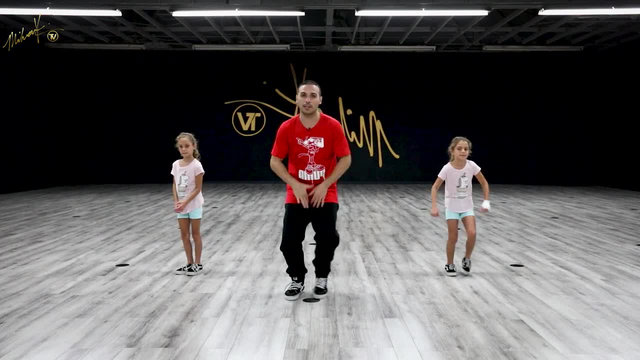 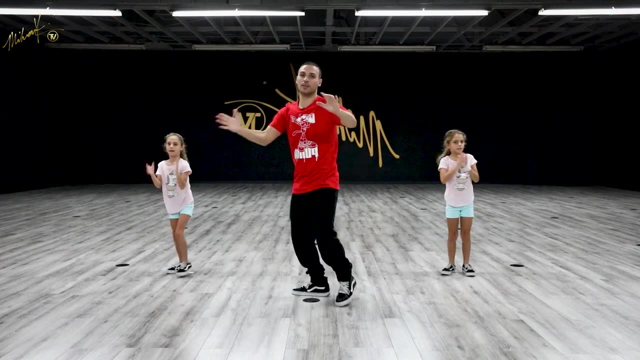 okay, Here we go. Five, six, seven, eight. Go one, two, three, four, five, six, seven, eight. Go one, two, three, four, five, six, seven, eight. Go one, two, three, four, five. 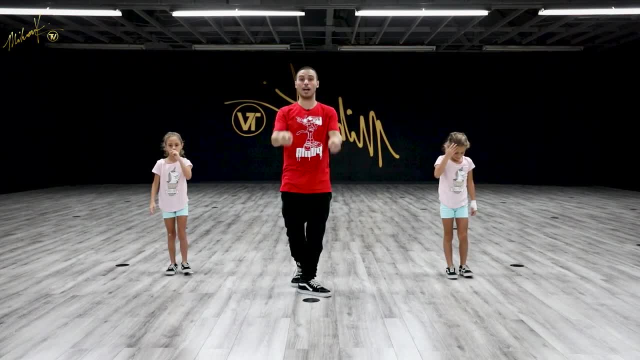 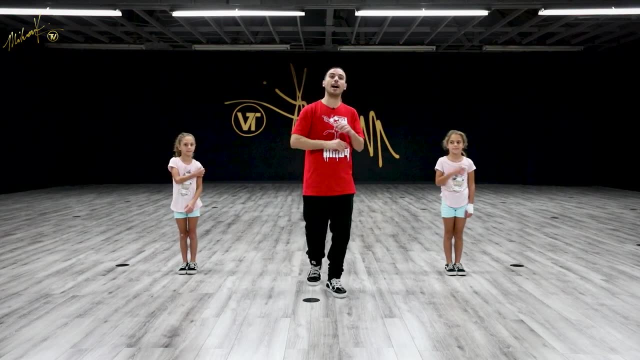 Five, six, seven, eight. Awesome guys, let's try it with music. All right guys, let's do it with music together. I'm gonna count you guys in Here. we go you ready? Five, six, five, six, seven, let's go. 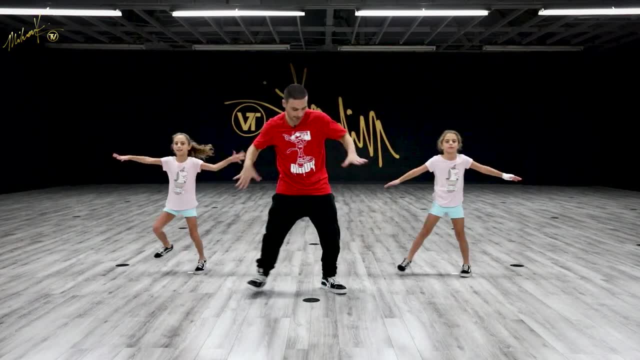 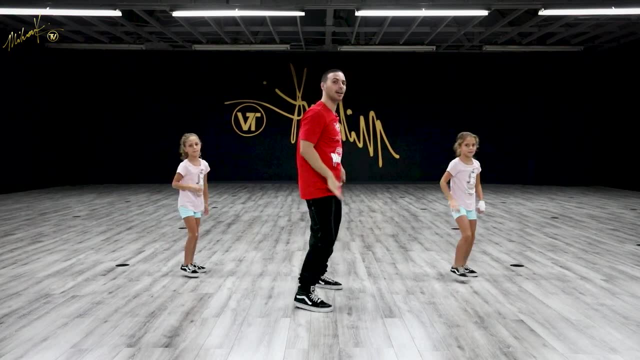 One, two, three, four, five, six, seven, eight. Go one, go two, go three, four, five, six, seven, eight. Good, let's do it again. here we go Five, six, seven go. 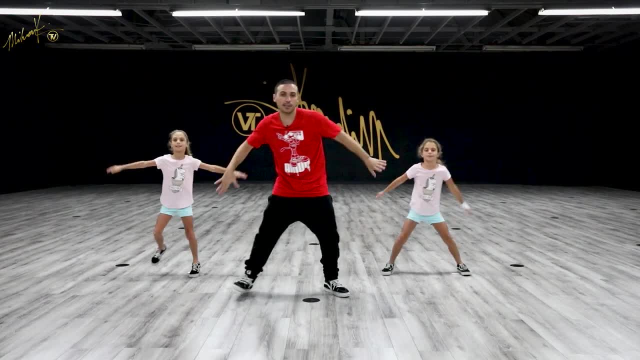 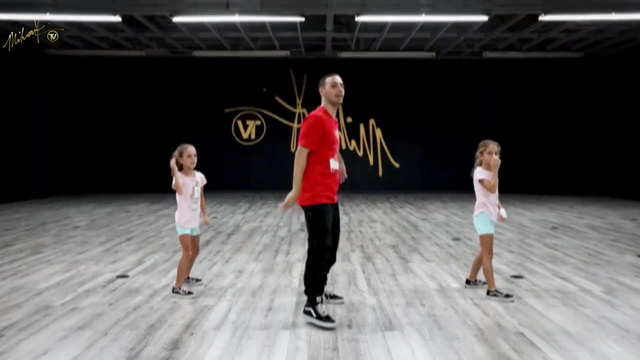 One, two, three, four, five, six, seven, eight. Step: one, two, three, four, five, six, seven, eight. Nice, All right guys, here we go, let's move on. So we ended here, right. 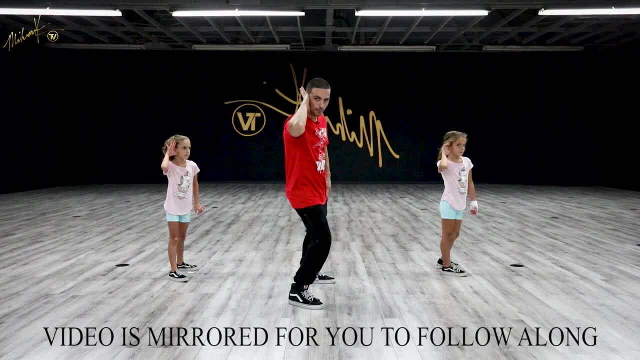 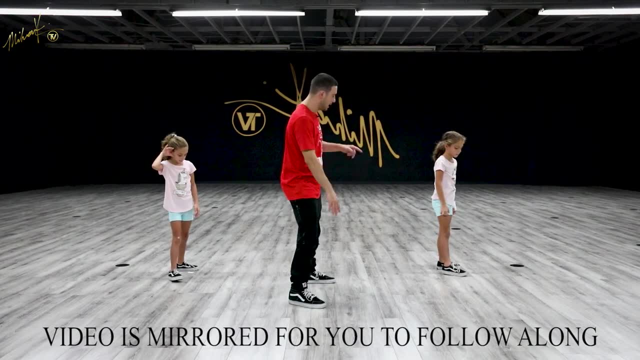 We leaned over, we went up down, up down, All right. so this move's a little tricky. We're gonna have to turn our body and face the back, So what I'm doing is I'm keeping my left leg in place. 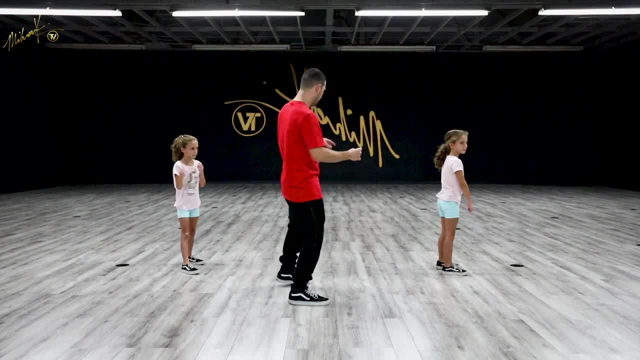 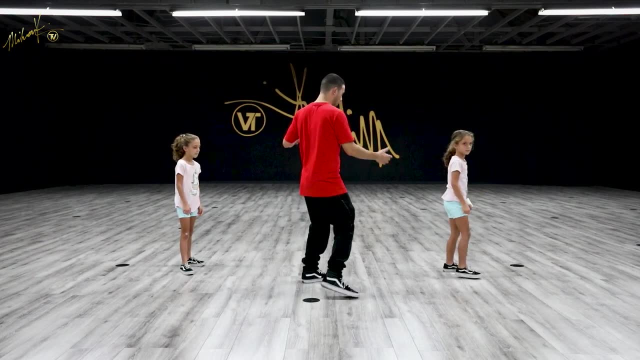 and only moving the right leg. So let's just watch once I'm going up, down, up down. Good, come back again. So again, you wanna keep your left leg there. Don't move your left leg. Your left leg is not gonna go anywhere, okay. 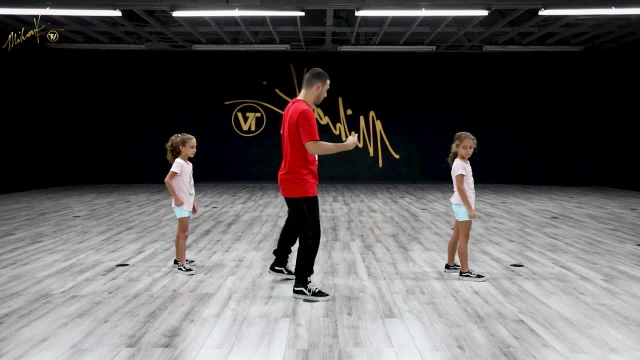 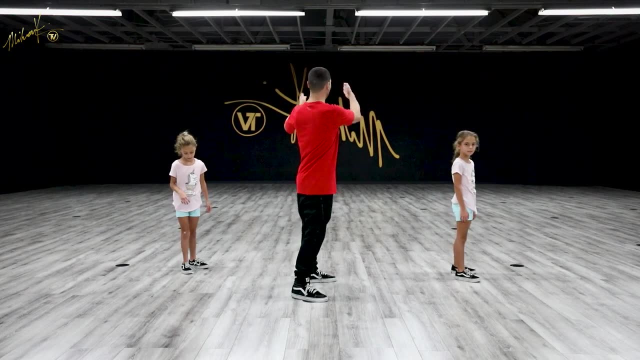 It's gonna be your right leg, But you wanna use that left leg as you're turning your body to turn your leg with you to be able to face the back, okay. So we got four counts to face the back. We have to bring our bodies. 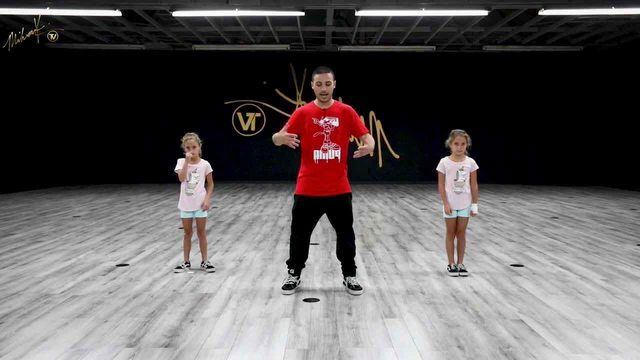 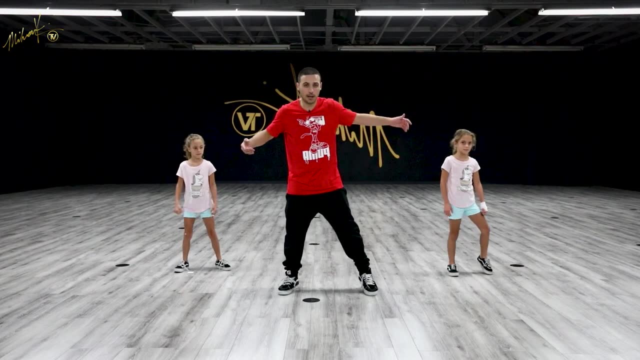 Girls, let's face the front one second, yup. Let's just show you guys the body. What you're doing is you're going up on one leg and then kind of dropping back down, bending your knees, And then up, drop. 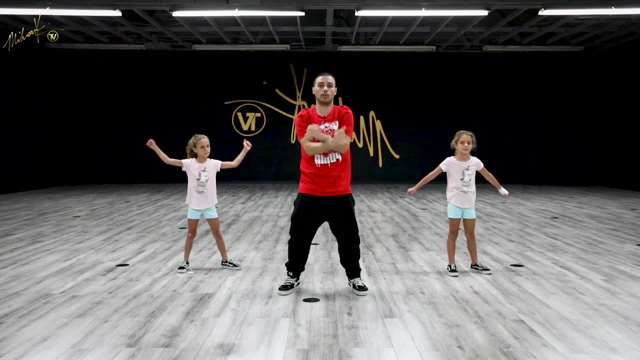 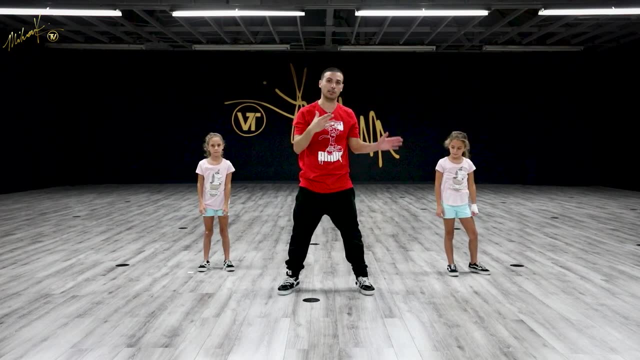 And then your arms are swinging the same swing you were doing. right, We're gonna go up, down, up down. okay, Now, every time you're stepping, it's a little touch that's gonna turn you: Touch up and step stop. 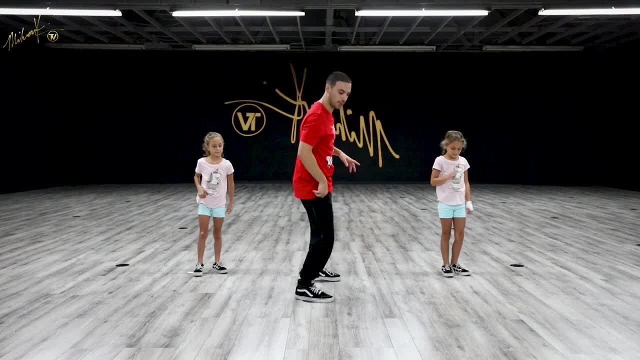 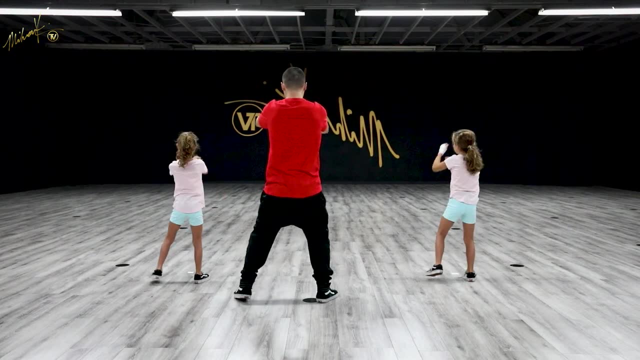 Good, so that's where we wanna get, okay. So let's do that a couple of times from here. You went seven, eight. We're going up and down, up and down. Good, one more time. I know it's a little tricky to not move that left leg. 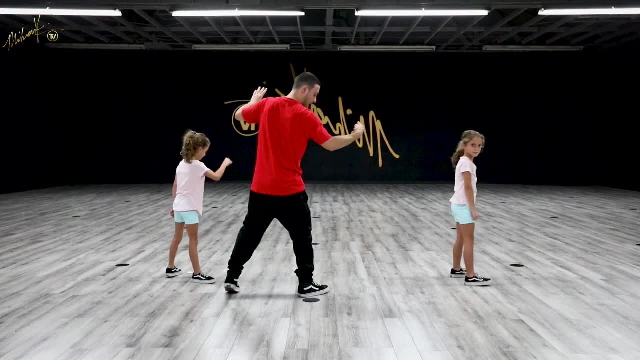 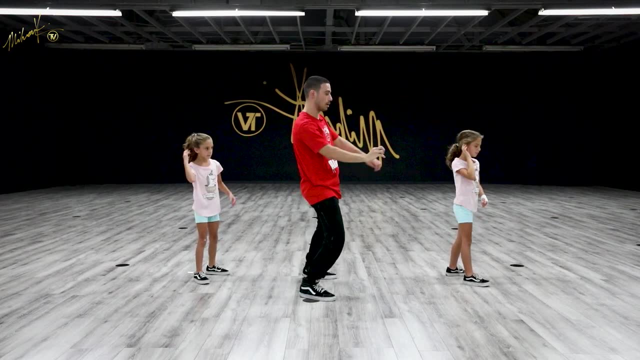 but you wanna make sure it's there and just turn it as your body's going, okay, So you don't really move from your place. Let's go again. Seven and down and down. We're going one and two, three and four. 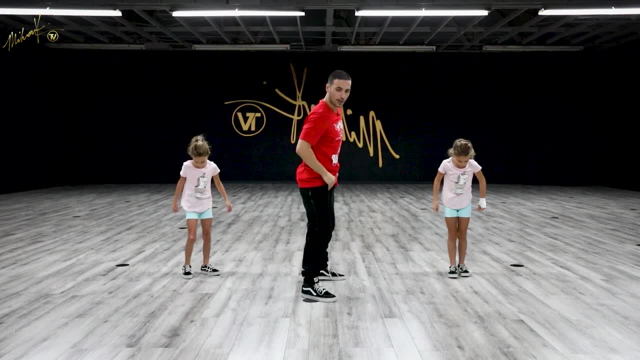 Good, let's do it one last time. Girls go back to your spots. Here we go. Five, six, seven, eight We're going up and down, up and down. Good, one more time. Eight go up and down, up and down. 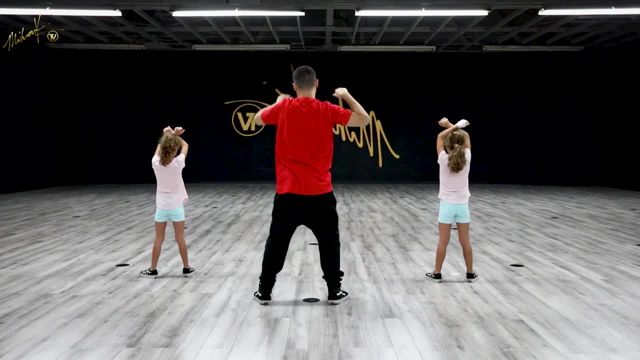 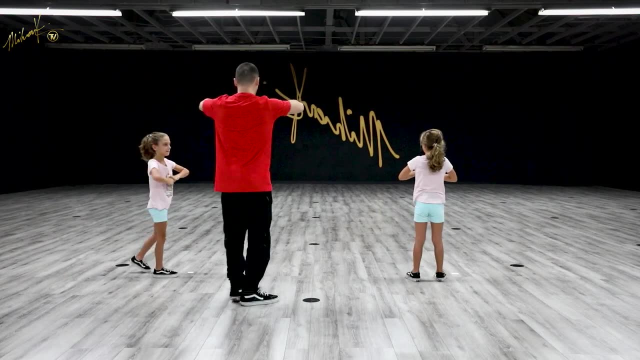 Good, I'm gonna stay backwards as I explain this, because it's easy. We're just gonna slide over one, put the feet together and the arms come here, just like that whoop, And then we're gonna go to the other side. 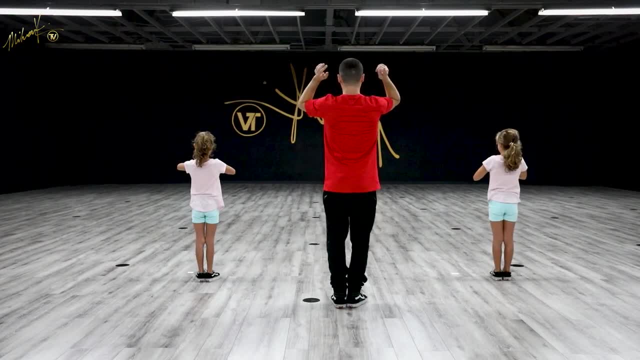 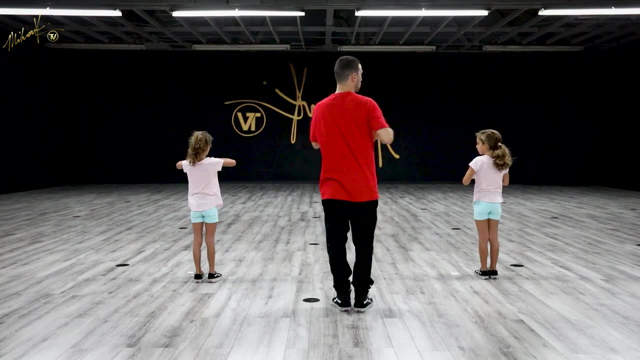 Slide whoop. Okay, let's do that again. Remember, you're facing the back. now Six, seven, eight, Go slide and hit, slide and hit. Good, I'm gonna show you guys, the slide Girls. you guys still face backwards. I'll face front. 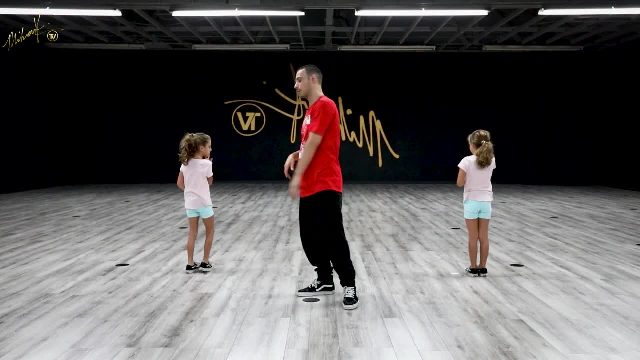 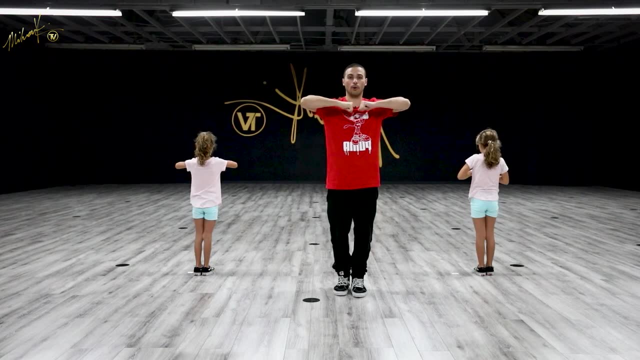 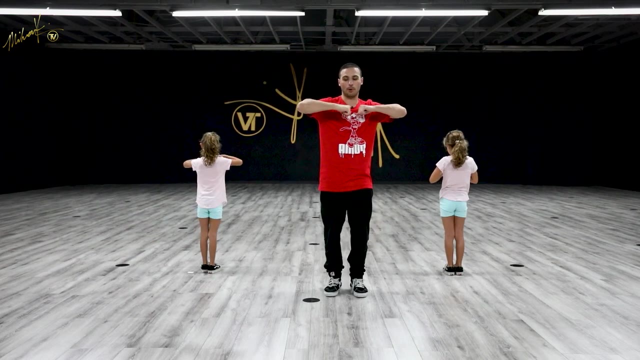 So, just so you guys see my arms with the slide, we're still gonna go to the right side. Six, seven, eight, Go. one and two, three and four. Again, five, six, seven, eight, Go. one and two, three and four. 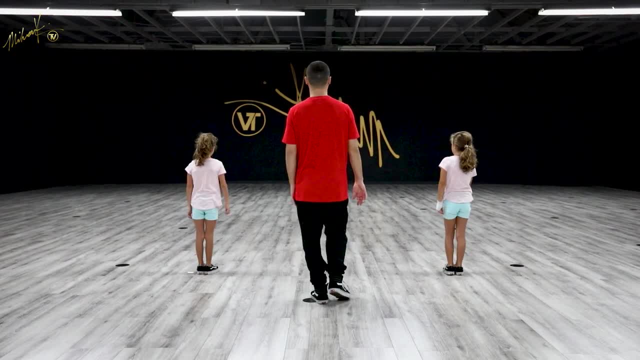 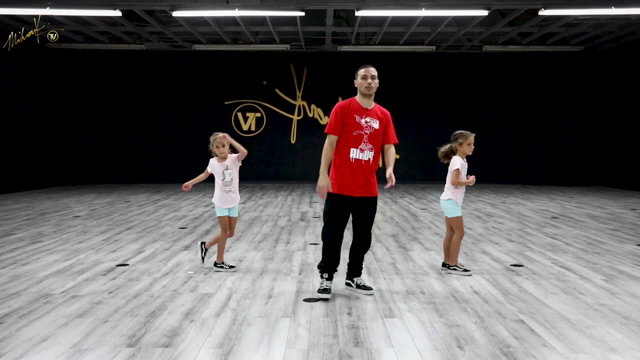 Perfect. So one more time, all of us facing the back, Here we go. six, seven, eight Go one and a. two, three and four. Bring it back. So remember, when you're doing the arms, keep those elbows up. 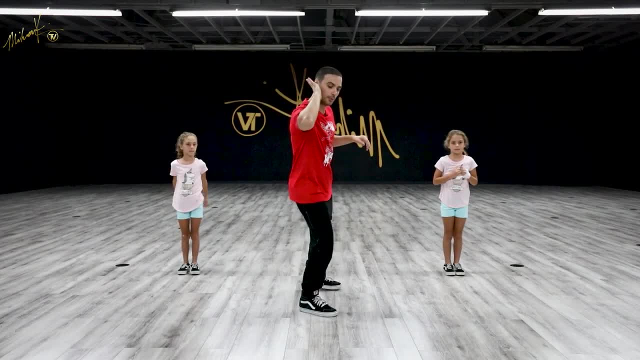 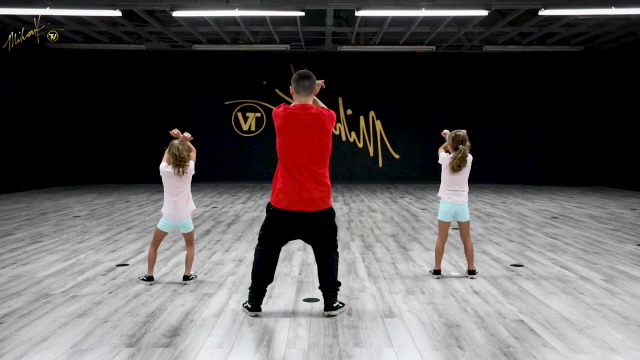 You wanna have a straight line. You don't want it to be broken like that. Let's go from here. Here we go. six, seven and eight Go up and down, up and down, Slide together, slide stop. 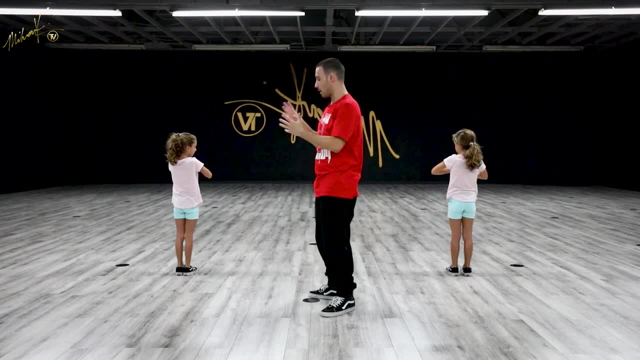 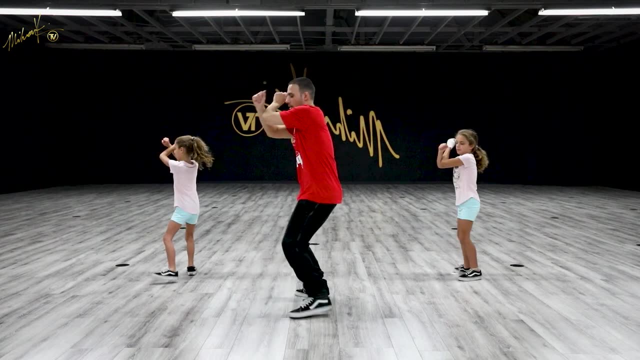 Good, from here we're gonna go right into the same exact move to turn our body back to the front. So here we go, let's show them: girls, Six, seven, eight, We're going up and down, up and hit. 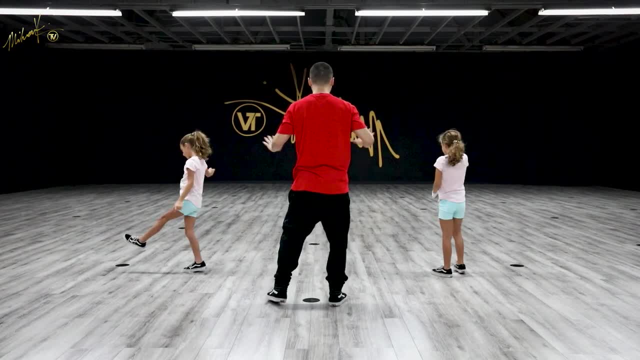 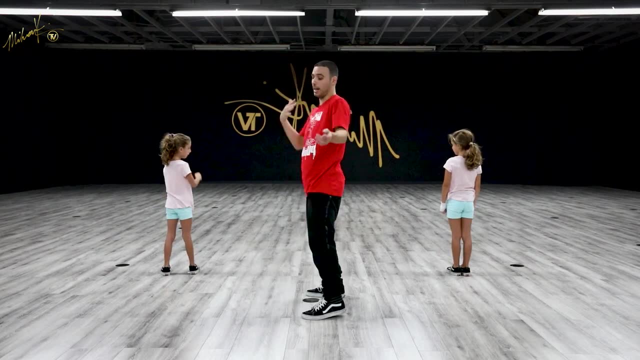 Good, now we're facing the front, Okay, so let's try it one more time. Same exact move, don't change anything. Left leg stays here again. The right leg does the movement. You're still going up and down. Make sure you go down and the way you're gonna go down. 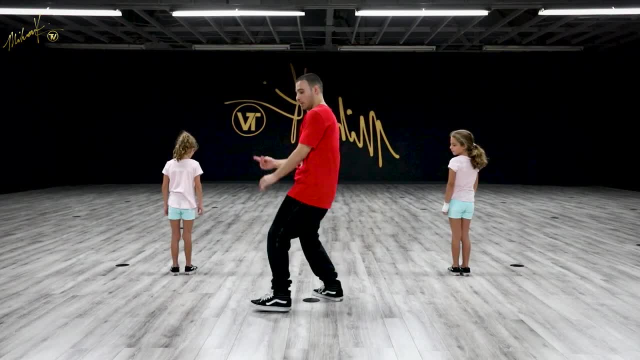 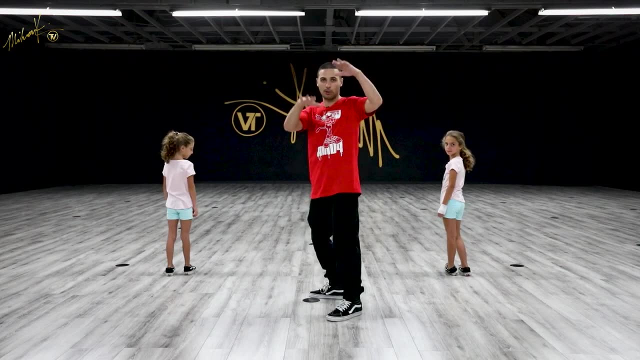 is by bending your knees. So there's a level change. Whoop drop, whoop drop, Even though I'm going up only on one leg, but I'm still dropping on both legs to give you a level change, okay. 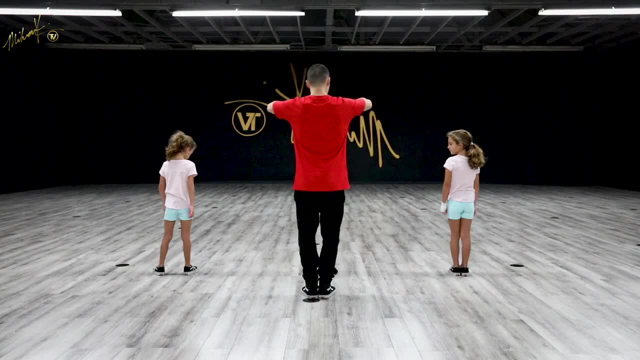 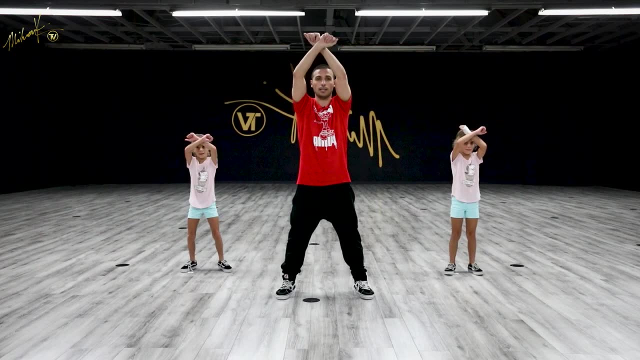 One more time. girls, you ready, Feet apart? Oh no, feet is not apart. We just finished here. Good job, Soph. here we go. Six, seven, eight, Step out and drop out and hit. 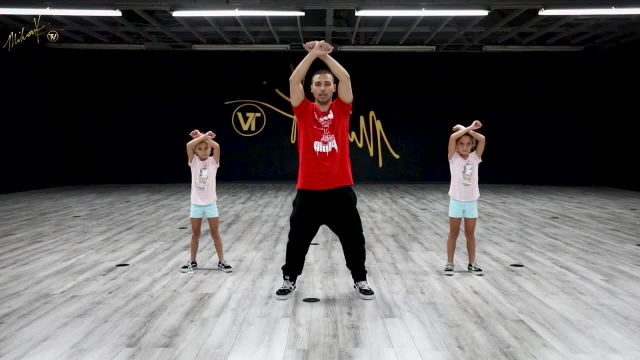 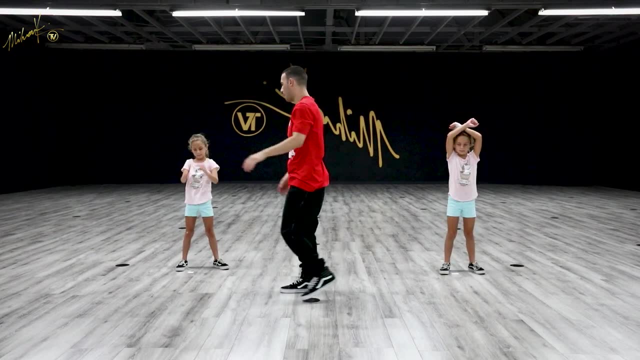 This is the last. one is the one you don't need to actually drop. You wanna stay here because you're gonna go right into a slide, So step and drop, step and stay. okay, One more time and we're gonna finish it up. 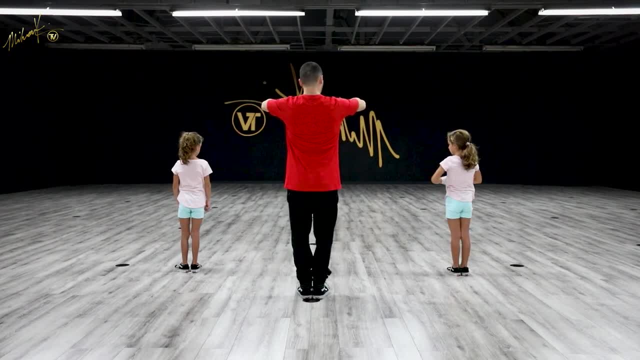 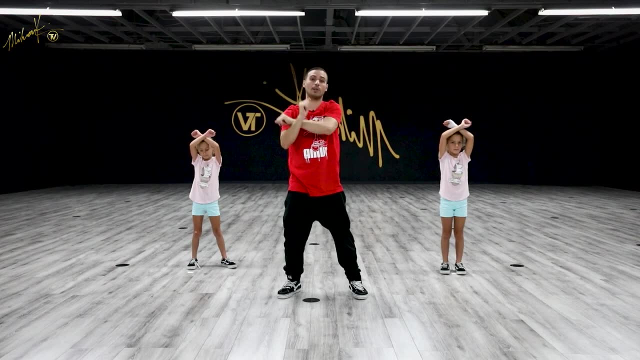 We're almost there. here we go. Five, six, seven- let's keep the arms up, girls. Here we go, elbows up. Seven, eight. we're going up and down, up and down. Now we're gonna do four slides really fast. 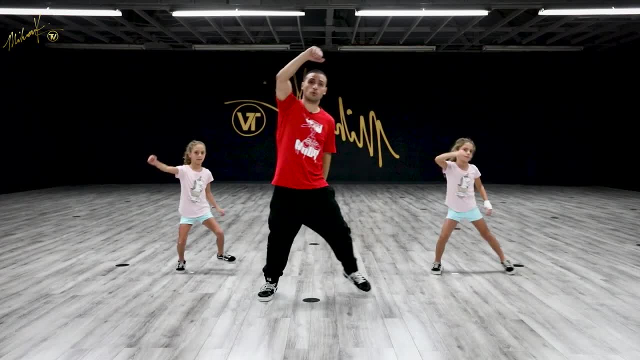 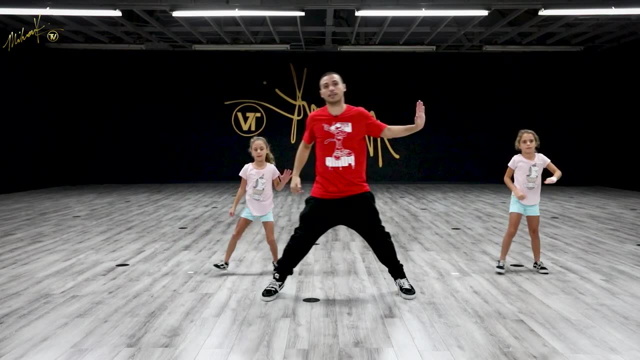 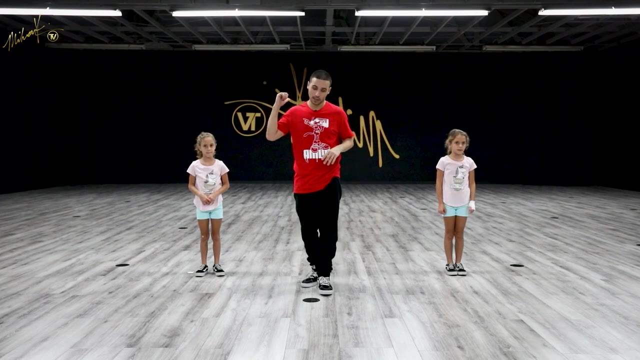 We're gonna go Slide, slide, throw the arm, throw the arm Again. five, six, seven, eight. Go slide, slide, throw, throw. Good, so you have four slides in four counts, which means you gotta slide every single count. 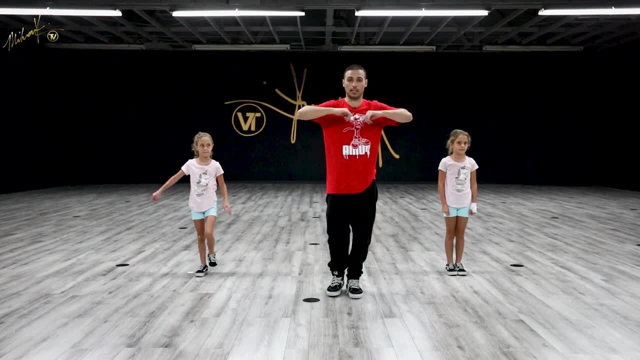 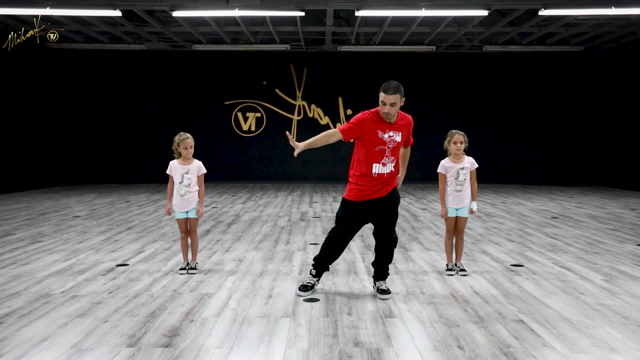 The slide before that was a two count slide. We were going one together, slide together. These are single slides, so don't complete sliding the leg in or you'll be late. You'll go one right into the next slide. 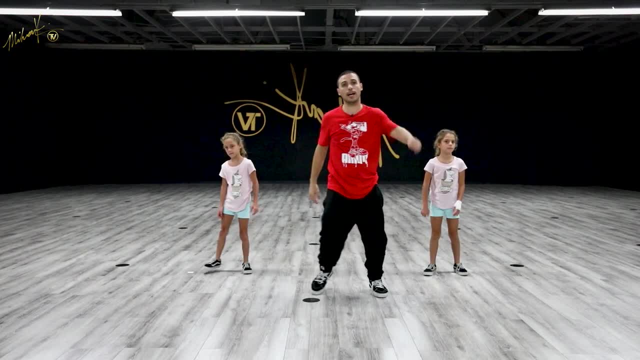 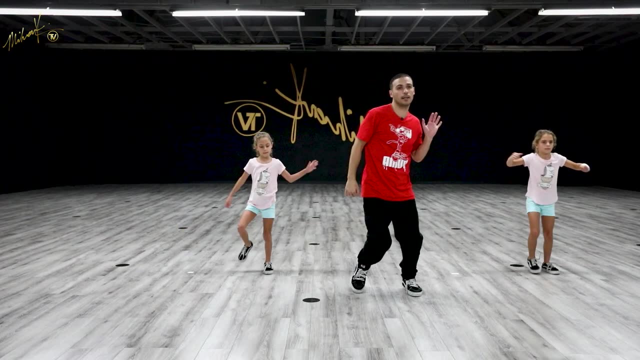 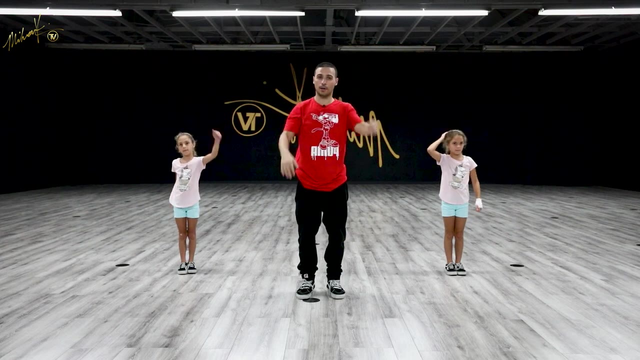 Two: right into the next slide. Three: right into the next slide Four: good, Let's do it together. girls from the slide Six, seven, eight, Go slide, slide, slide, slide. Good, again, you're gonna go push, push up up. 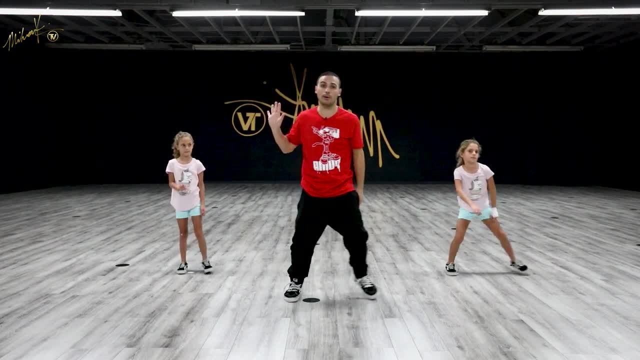 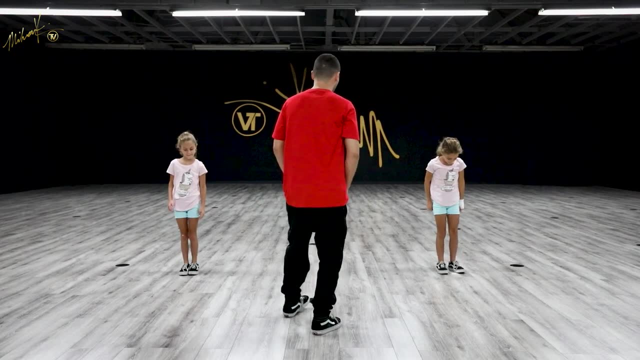 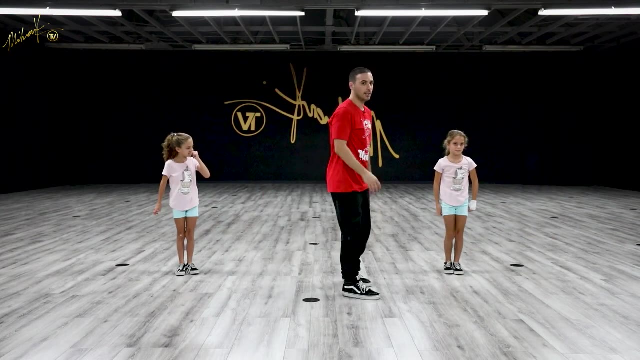 Again. five, six, seven, eight, Go slide, slide, boom, boom. good, How does it feel, girls? Let me see it. Just the slides. five, six, seven, eight, Seven, eight, go push, push, throw throw. good, good job, all right, so that's the routine. 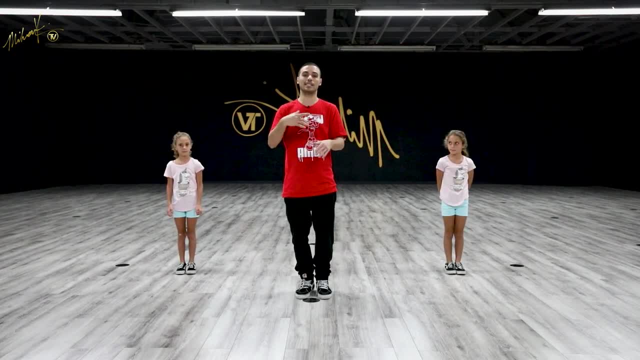 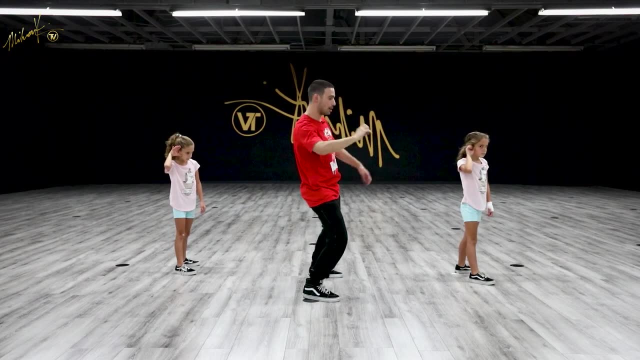 that was it. four, eight counts. we're done with the full routine, so let's take it back, go from the second section and then we'll take it back and go from the top. so we went seven and eight. we're going up and down, up and stop. remember, this is the two count. 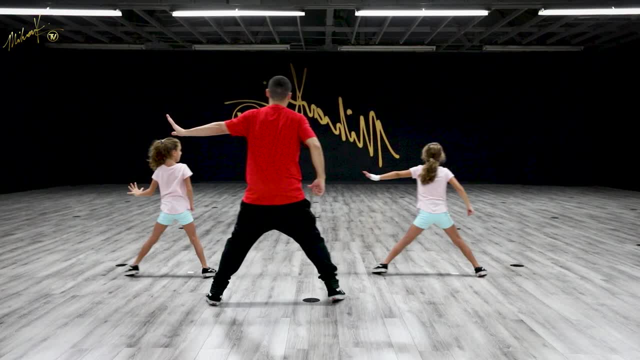 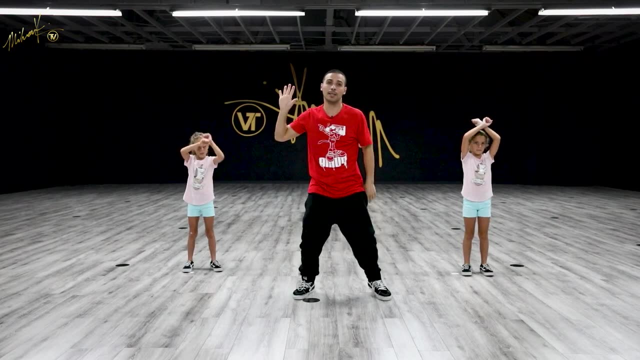 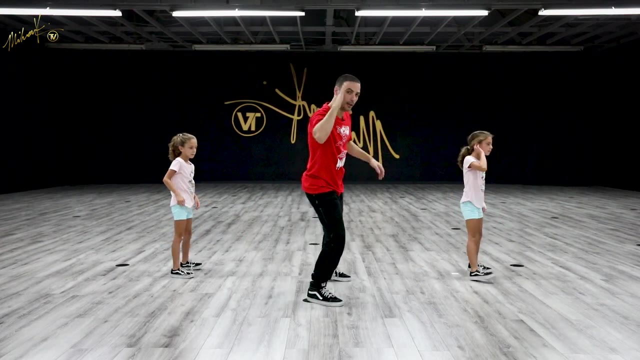 slides five feet together, seven and eight. now one and two, three and stop. this is the single slides: slide, slide, slide, slide. awesome. now I'm not going to stop, we're going to go through that. here we go: five, six, go, seven, eight, go up and down, up and. 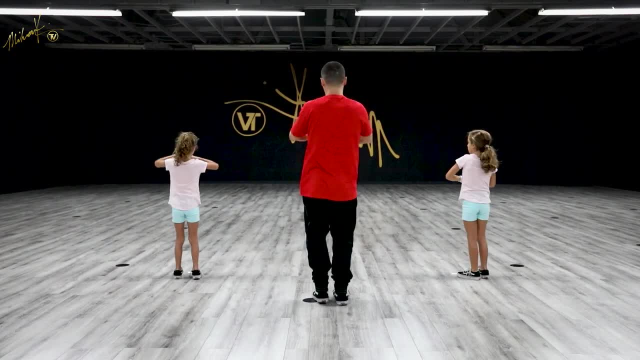 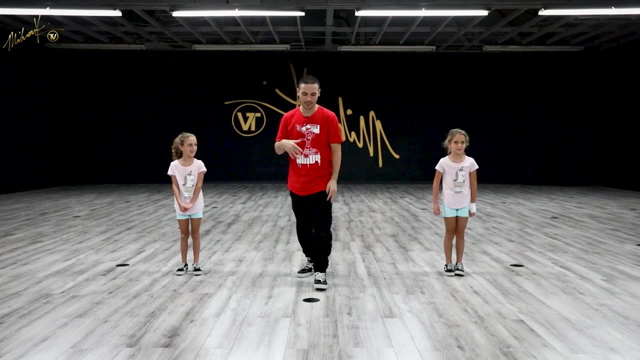 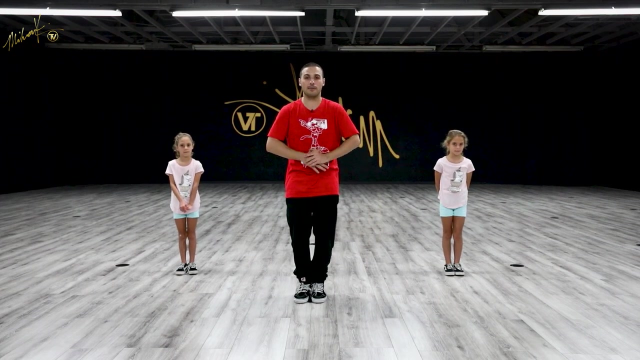 down, slide and together slide and together. up and down, up and down, Go, slide, slide, slide, slide. let's walk it slow, okay, just to make sure we're all on the same page. feet together, feet together, feet together, five, six, seven, go and one. 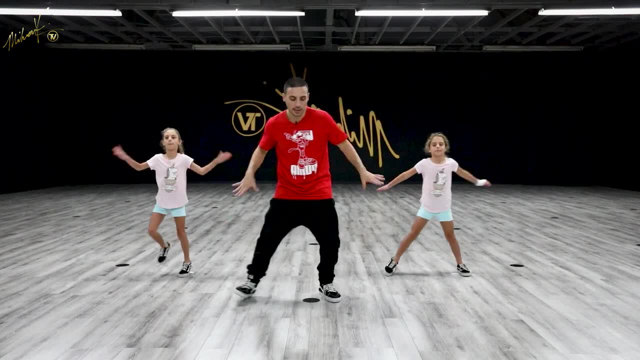 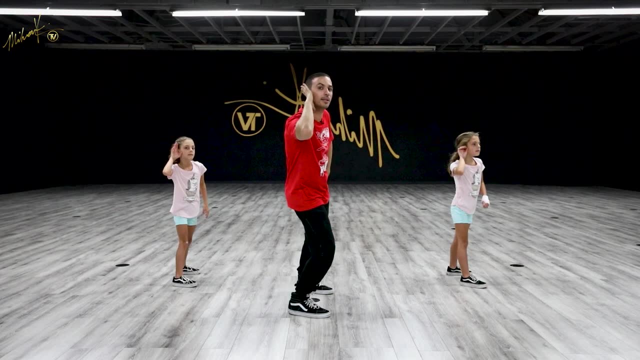 two, three, four, five, six, seven, eight. step one, two, three, four, five, let's do six, seven, eight. go up and down, don't move the left leg. slide, step, slide, step. 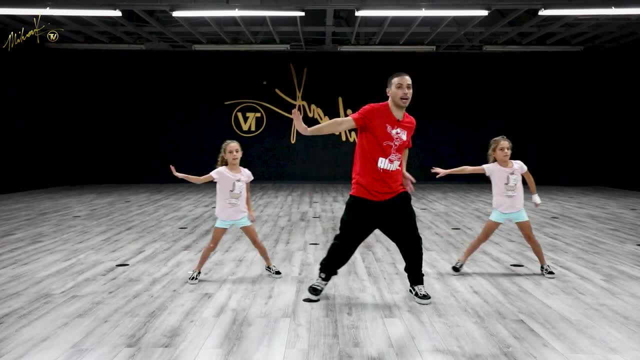 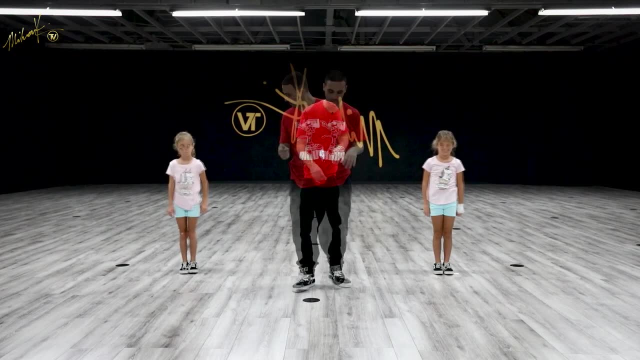 go up and down. up and down, go slide, slide, slide, slide. good job, let's do that again. let's speed it up a little bit. here we go, let's go back to our places. five, six, seven. 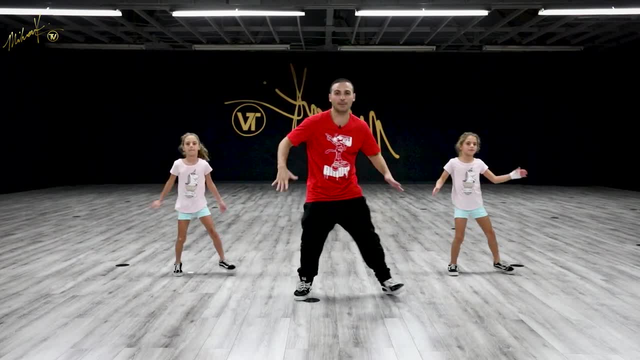 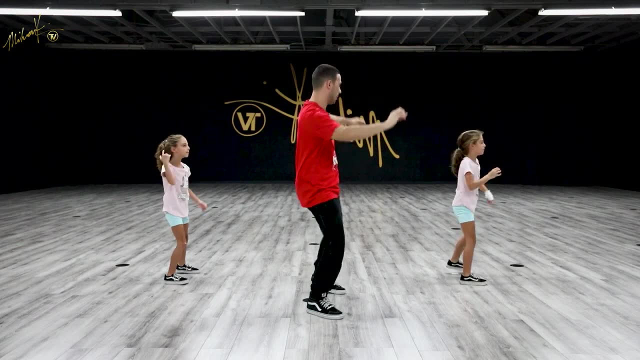 eight. go one, two and three, four, five, six, seven, eight. go one, two, three, four, five, six, seven, eight. go up, down, up down and slide together, slide together.